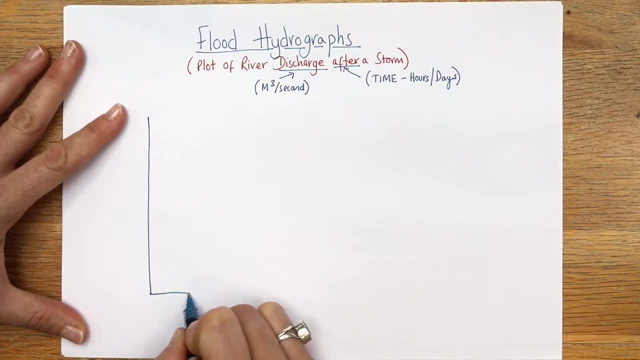 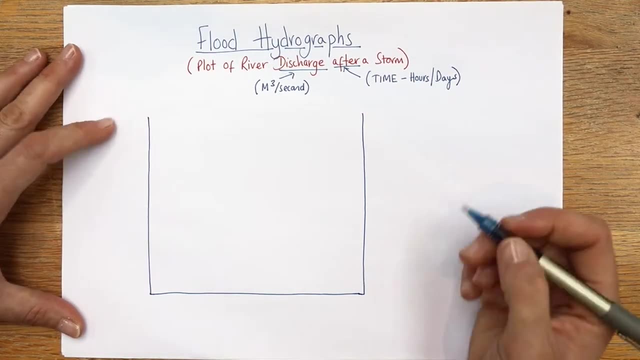 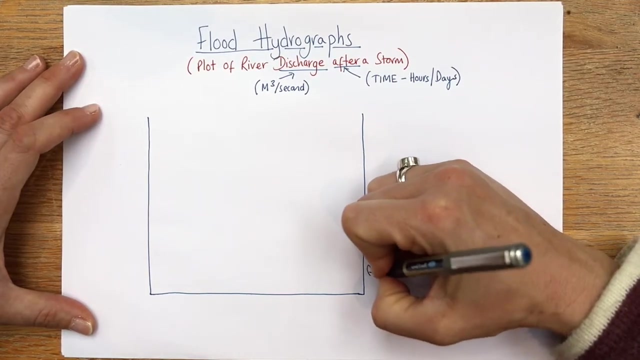 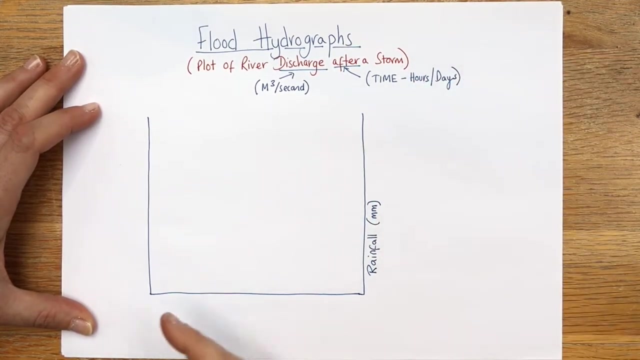 best straight line, and then another one along here, and then another one down here. Don't need a ruler, you can just do it very slowly and carefully. Okay, let's label our axes first. so on this side we're going to have rainfall, and that's measured in millimeters. On this side we're going to have time or at. 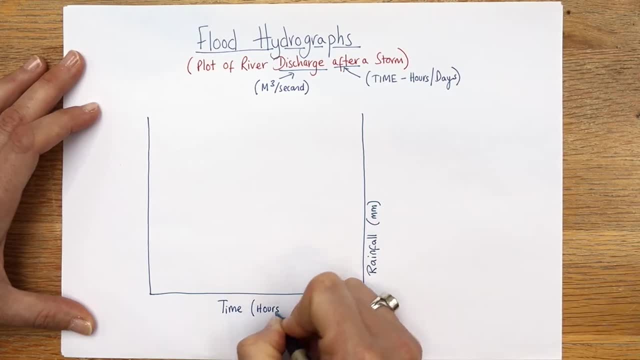 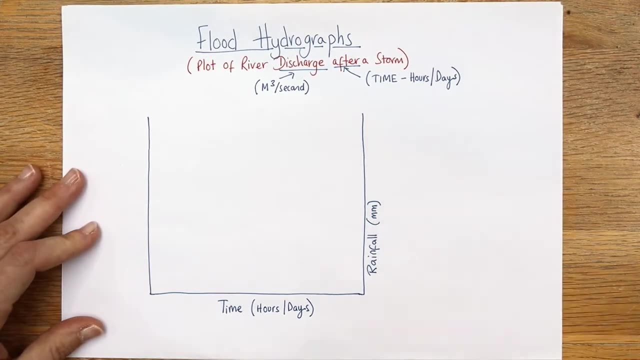 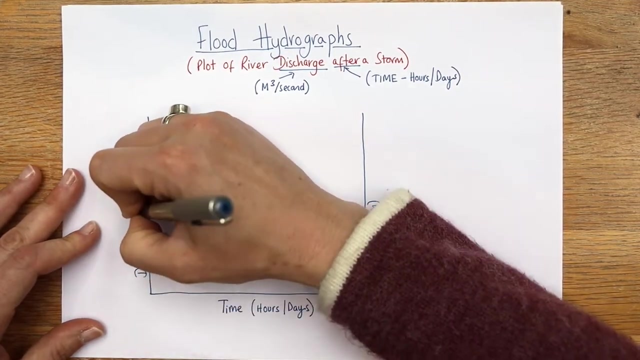 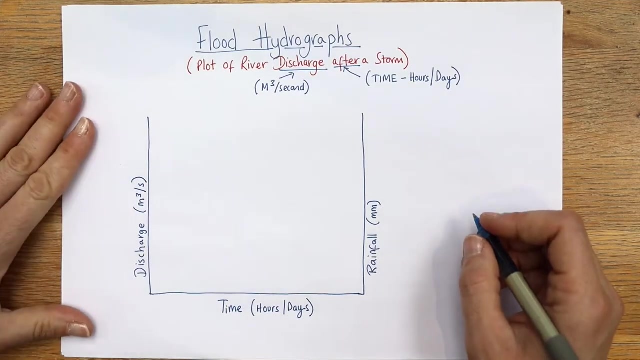 the bottom rather- and remember that's hours or days depends on the graph you're given- And then on this side, this is where we measure the discharge. so how much water is coming out of the river Discharge, and that is in meters cubed per second. Okay, now the base flow of the 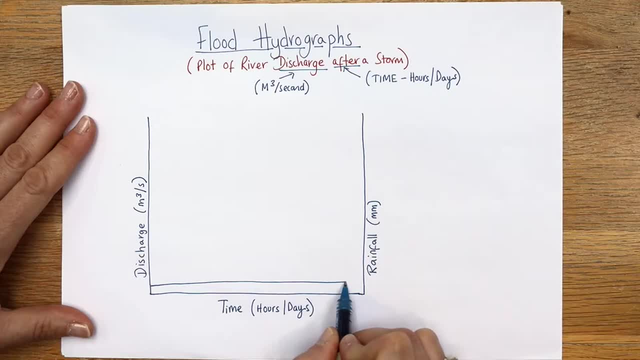 river. just going to put that in first. let's pop it there and we're going to label that base flow. This is what the river does under normal circumstances and normal amounts of rain. it's steady, there's not too much water being pushed out, there's no flood event. 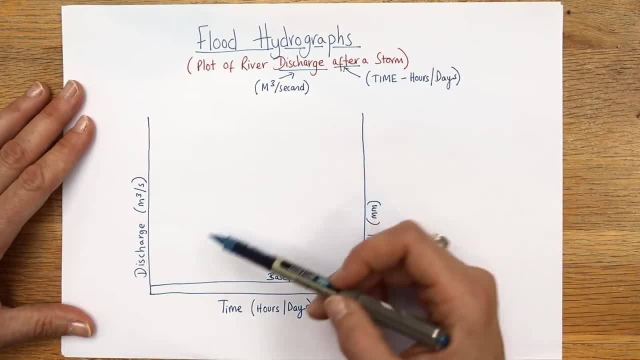 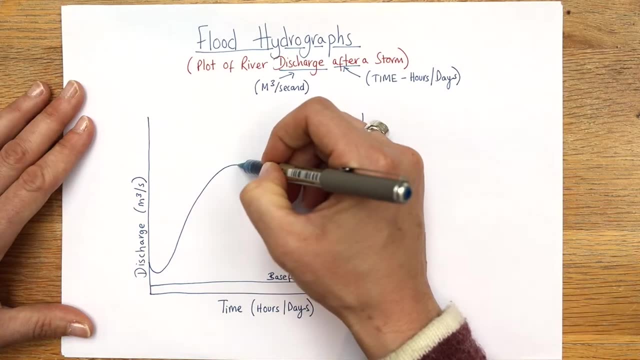 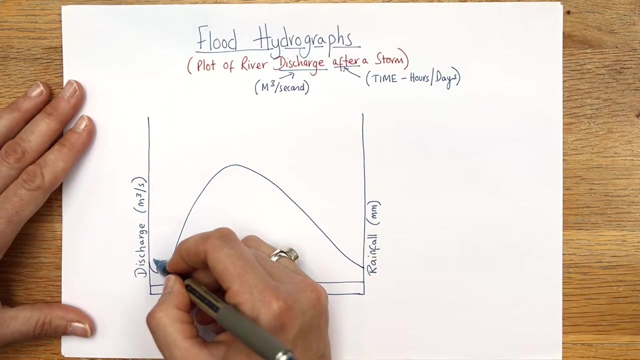 Now we know that there's been a storm, so this is going to look a bit different now. and what happens if you watch me first and then copy yourself, is you get something a bit like this: Okay, now the rainfall, I'm going to draw the bars. it's a bit. 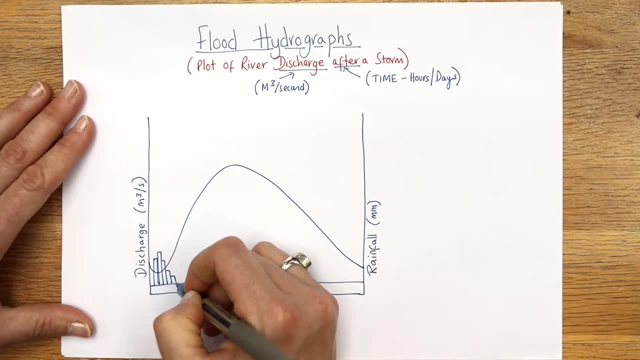 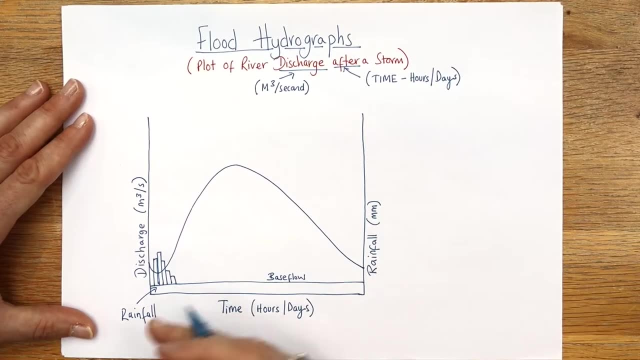 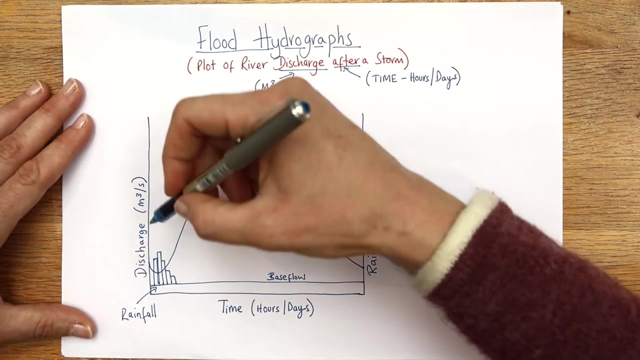 like a climate graph. There we go. so we've got our rainfall, our bars. Often the rainfall will happen. for how many? let's say. let's say a day, that's a lot, but you know, whole day of rainfall, whole night of rainfall, and there is a lag time between the highest. 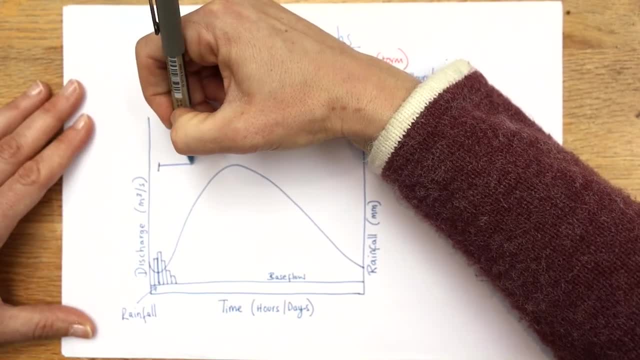 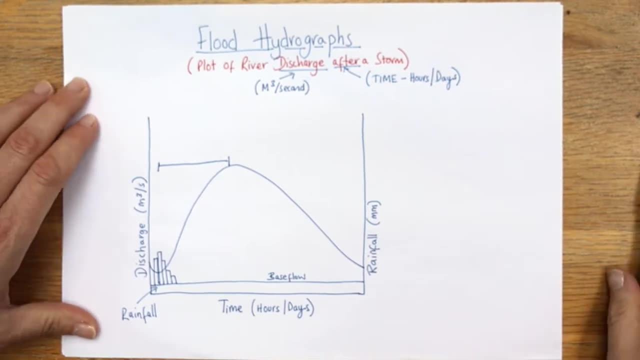 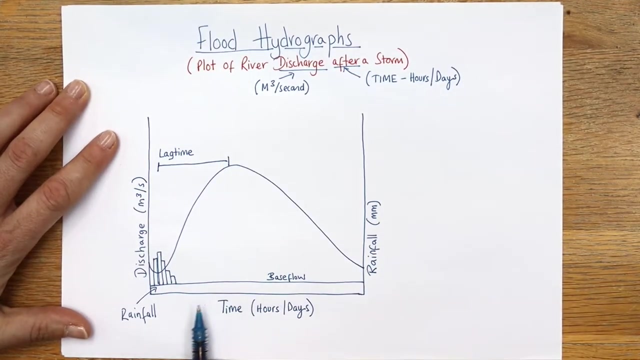 point of rainfall- and I take over here- and the highest discharge. remember we're measuring discharge from the river. Now that is called the lag time. Okay, and the lag time here. I haven't got the exact measurements on here, but we could say it's two days, three days, and remember that the reason for that is water takes. 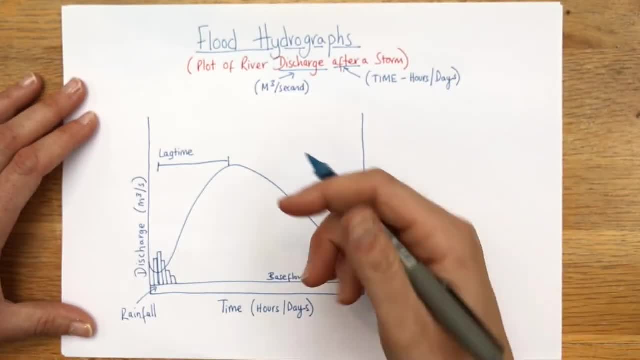 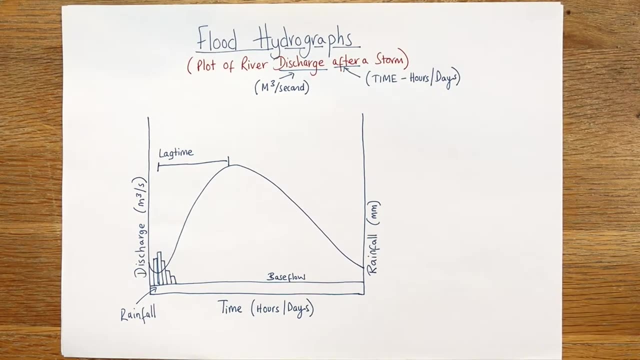 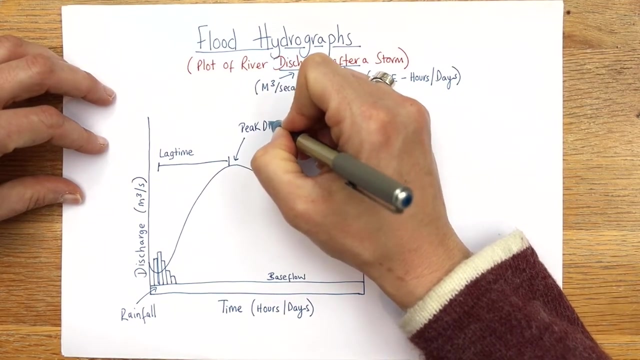 time to get to the river. it might be caught in trees. it might be soaked up in the ground, it could be. it could be many reasons why it's not exactly there yet. Okay, next up, we need to label our peak discharge, so that's like the biggest. 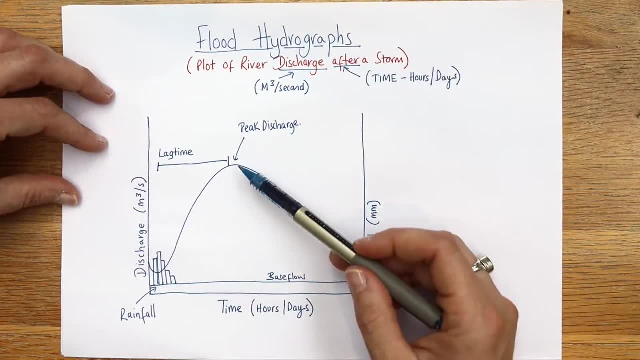 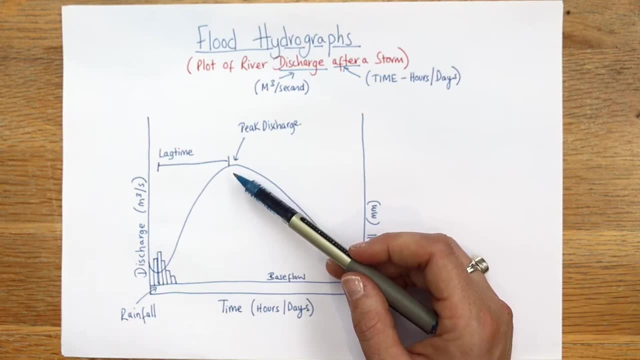 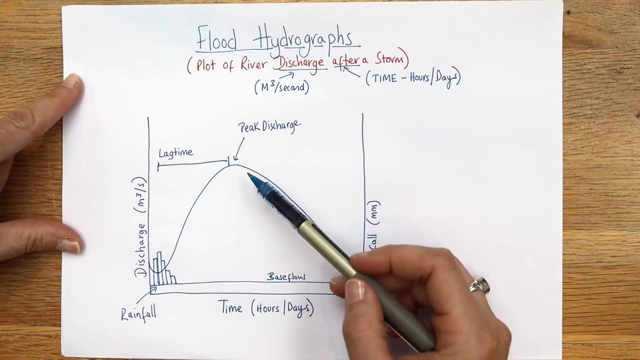 flow of the river. If this was a real flood event, that's where buildings would be being flooded, bridges would be destroyed. the river is running fast and high and flooding the surrounding area and then you can see it drops back down slower. so it rises quicker and drops back down slower Now. 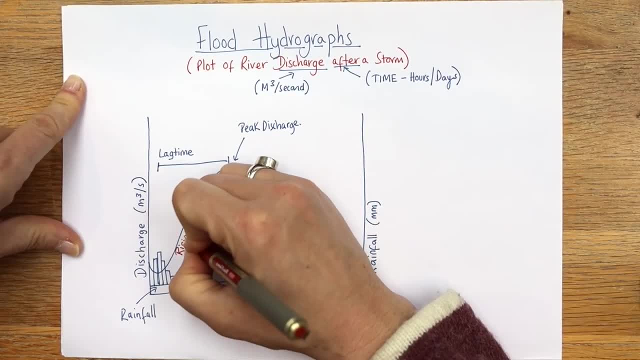 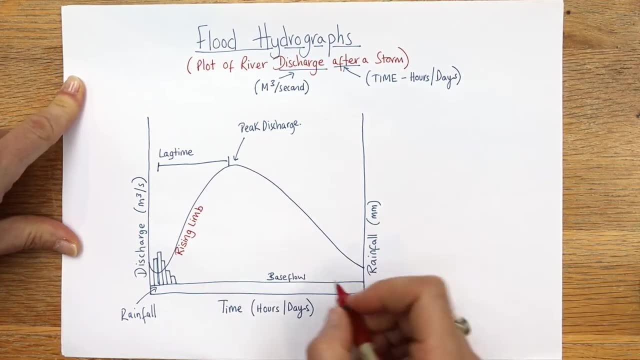 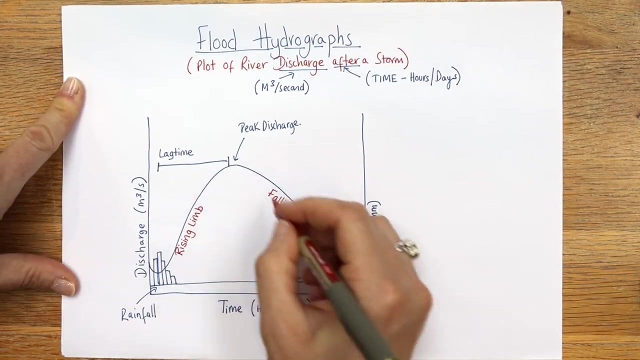 this one is called the rising limb. Limb is like a limb in your body. I'm not sure why they use that term, but that's what it is- the rising limb- and then this one is known as the falling limb. Now, this shape can be very different depending on how big the flood. 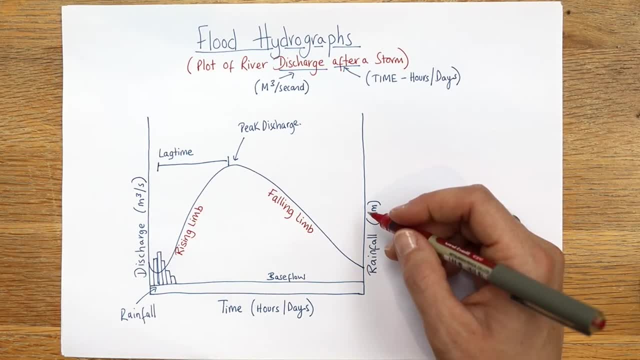 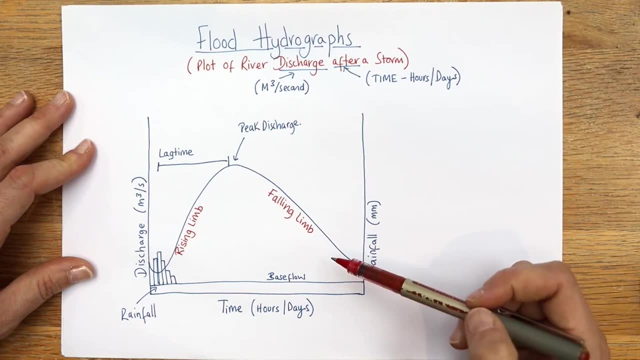 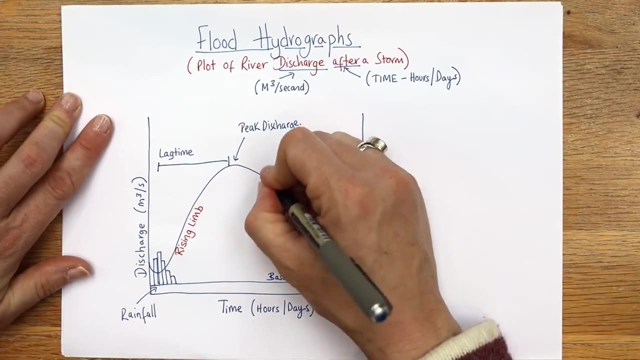 event is like how much rainfall has come over how much time. so if it's a flash flood, you'd expect to see a really big peak and then immediate drop, whereas if it was like prolonged rainfall, then it would be more steady. But basically, this line is showing you the volume of flow along the river. 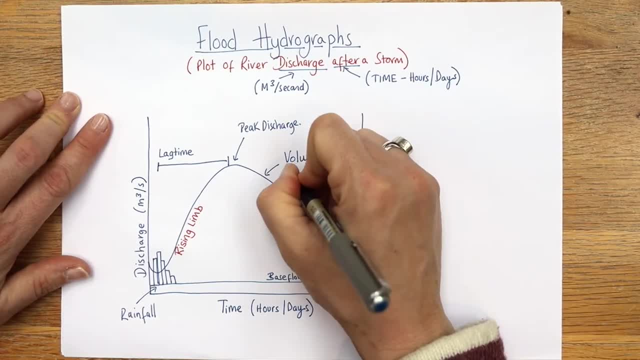 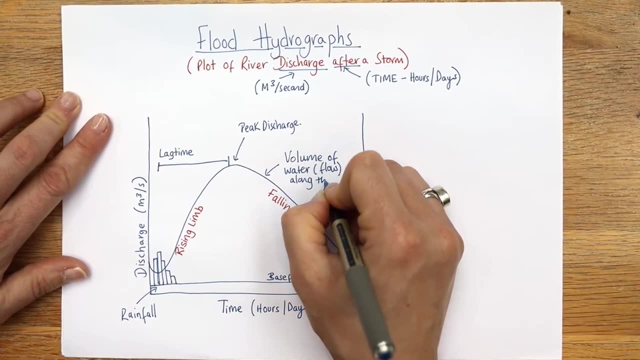 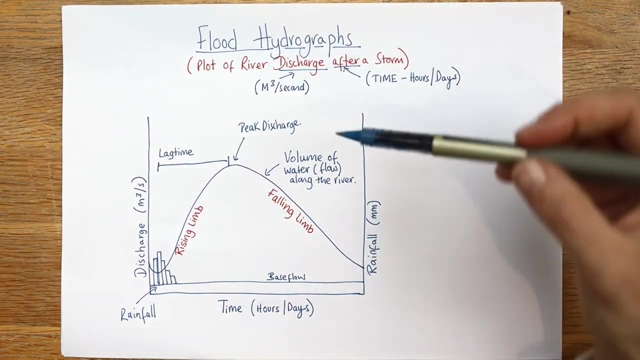 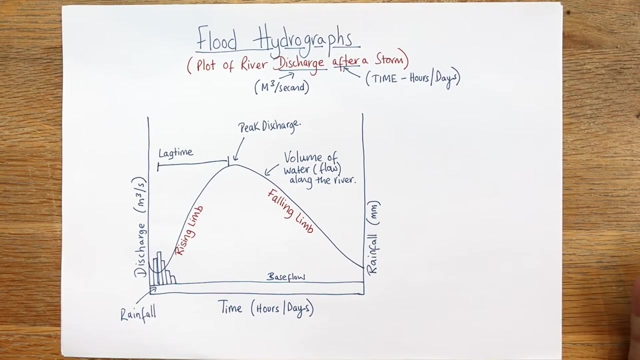 That's the line, That's the volume of water, or we call that the flow along the river. okay, so that's measured in in peak discharge. okay, We've got our rainfall measurement over here. we've got our base flow. we're doing really well. this is essentially what a 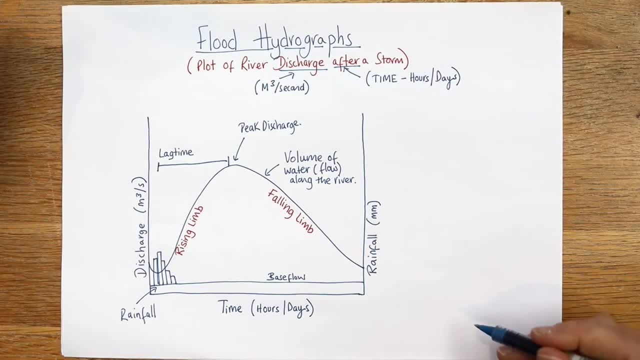 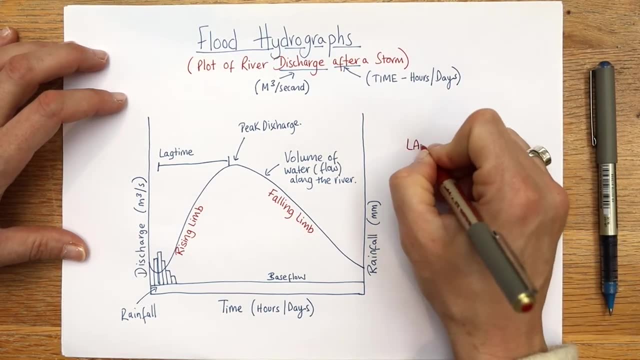 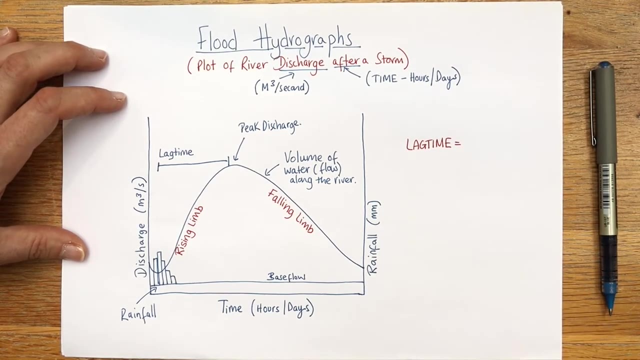 flood hydrograph looks like. Now we've just got to remember about the lag time and the base flow, so let's put those over here. so our big keywords. So lag time, which remember changes depending on if you had a flash flood where a lot of